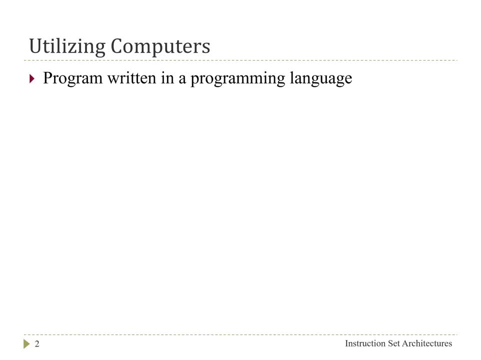 operation that we'd like to achieve, and these programs are written in some programming language. There are lots of different programming languages, but they all have a number of common features. So for a program language it generally takes on a somewhat natural language-like form. So 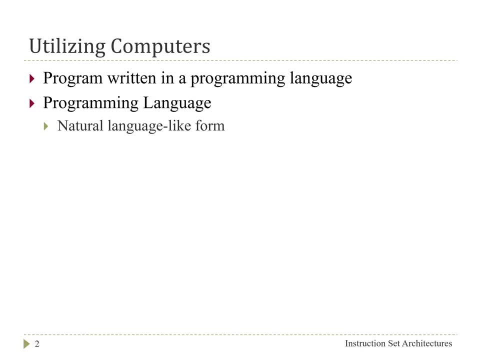 while it's not exactly like the languages that we speak and write, it does have elements that are similar to that that allow it to be relatively easily understood. Common programming languages have a number of similar structures that allow you to express the type of operations that you 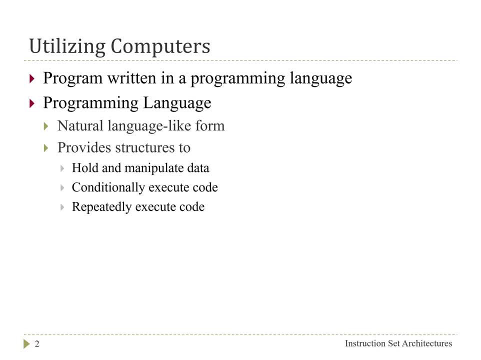 want or that you need to achieve your goal, And so these include the ability to hold and manipulate data and the ability to manipulate data. And so these include the ability to hold and manipulate data and the ability to manipulate data, And so these include the ability to hold and manipulate. 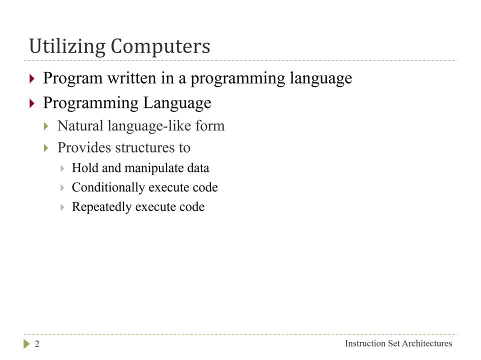 data, the ability to conditionally execute particular pieces of code based off of the state of some piece of data, and the ability to repeatedly execute a region of code. And then, once a program is written, another piece of software, referred to as a compiler, maps this. 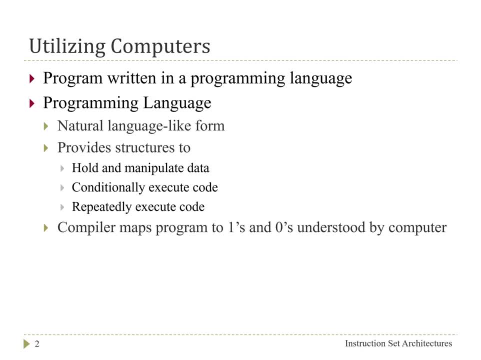 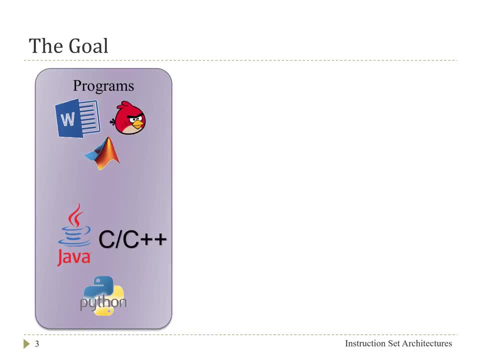 program into the ones and zeros that can actually be executed in digital logic, And so our general goal is to be able to have a set of programs. this can be different applications and they can be written in different languages, And we'd like to be able to take these programs that have been written. 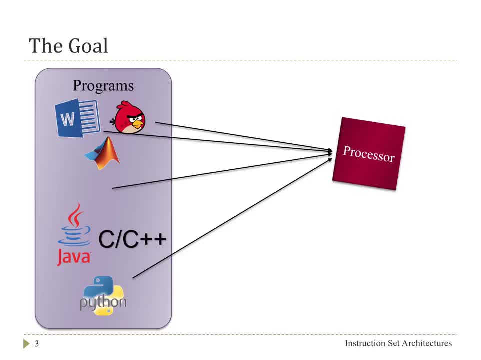 and execute all of them on a particular processor. And not only would we like to be able to execute them on one processor, we'd also like to be able to execute the same programs with very little, if any, modifications, on a different processor, And so the challenge is: how do we take programs that are 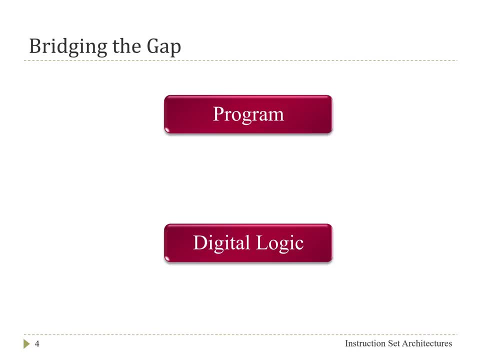 written once and essentially allow them to be executed on processors that could be very different, And so we have programs that have been written in the digital hardware for different types of processors And while, theoretically, we're going to be able to execute them on different processors, 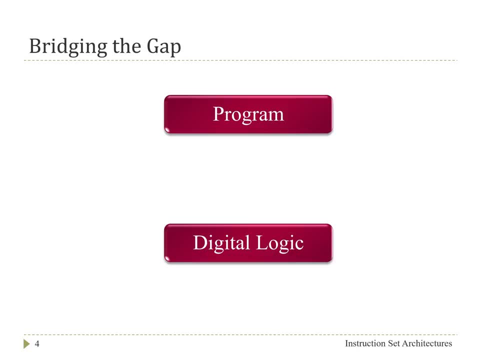 theoretically, we could create different versions of the programs for each different type of processor and its associated digital logic. In the end, with multiple different types of processors that have been developed over multiple generations or multiple years and decades, it becomes difficult and in reality, probably impossible, to support and maintain different versions of the program for. 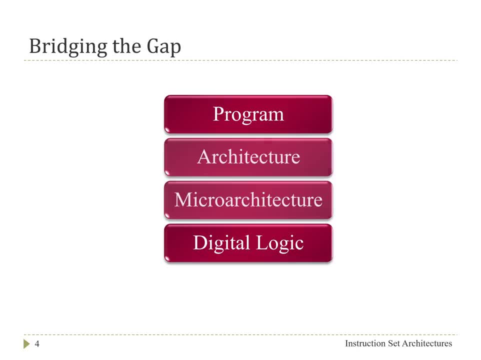 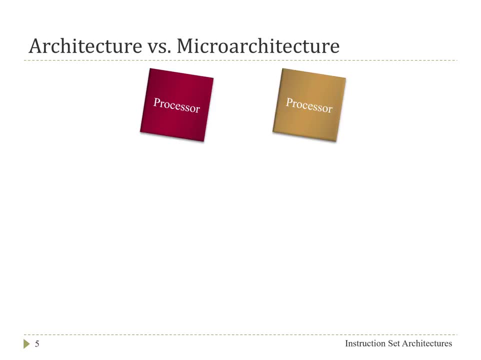 different types of processors, And so the way we bridge this gap is through a combination of what's referred to as the architecture and the microarchitecture. So to kind of explain what these are, we're going to start off with the two abstract processors that we had before. These processors are different processors with different 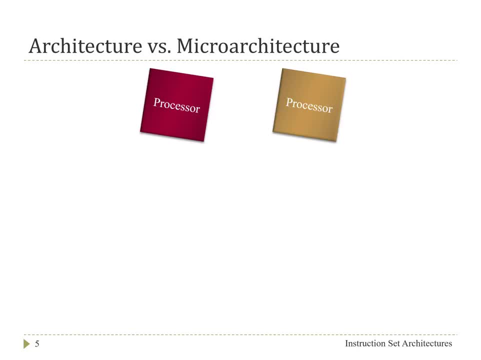 features and maybe different performance or power trade-offs, And right now these are abstract. but to make these a little bit more concrete, we're going to replace these with examples of three specific types of different processors that execute different types of instructions. So one is x86, which is used in Intel and AMD processors. 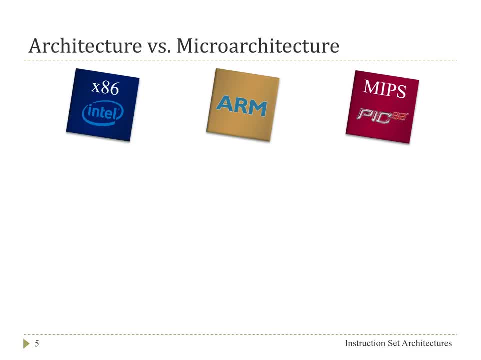 Another is ARM, which is used in a number of mobile and embedded environments, And then MIPS is another one that today is used in a number of embedded environments. And so each of these processors, for these different families, speak essentially different languages, And these different languages are essentially known as the architecture And so different programs. 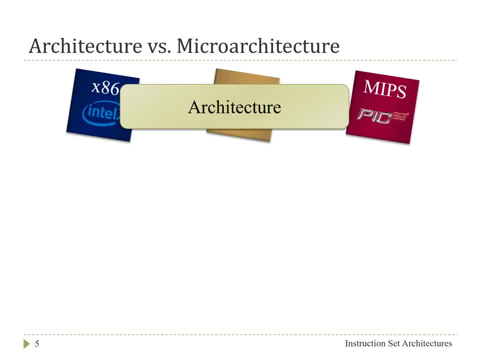 have to be compiled for different architectures. So you can have a program and compile it for x86 and also compile it for ARM and MIPS, And the x86 version should run any x86 processor but won't run on an ARM processor or a MIPS processor. 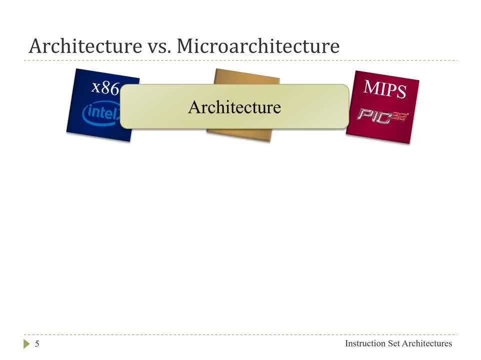 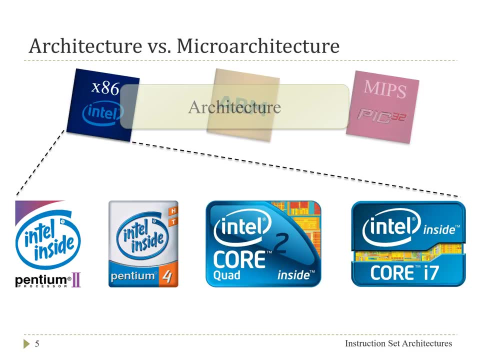 And then, within a single architecture or a single family of processors, we can have multiple different implementations of them. So, as an example, in Intel there have been lots of different generations of Intel processors. Here we're showing a few of them, from the Pentium 2 up. 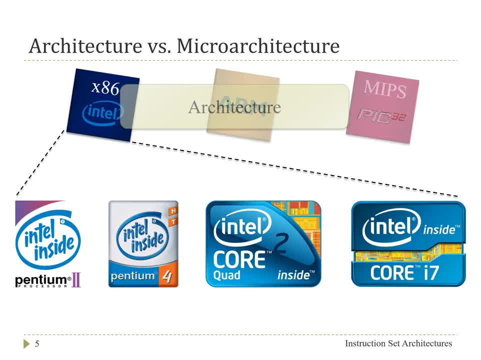 to contemporary Core i7 and similar lines of processors And any program that has been compiled for custom computer interfaces but not written for a particular architecture. so in this case x86 can execute on any of these processors, So a program that was written back. 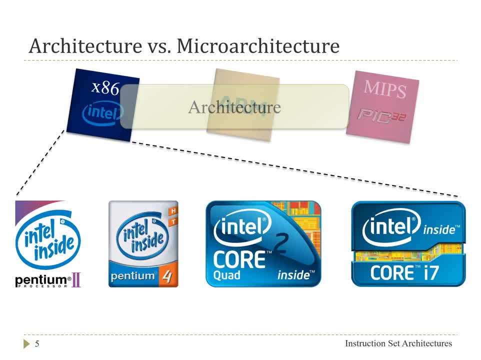 20 years ago that could execute on a Pentium 2, can still execute on contemporary Intel processors today, And there may be different trade-offs in terms of, or different benefits that these provide in terms of performance and power consumption, but they can all execute the same program, And so These 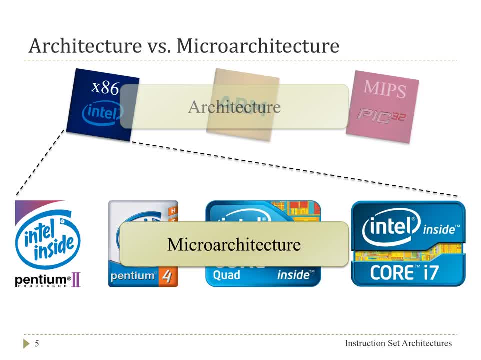 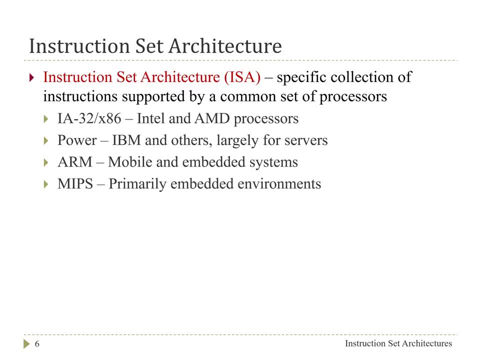 different implementations of the same ISA are examples of different microarchitectures. So the microarchitecture is the actual implementation of a particular architecture And so, when it comes to the instruction set architecture or ISA, essentially this is a specific collection or set of instructions that are supported by a common set of processors.